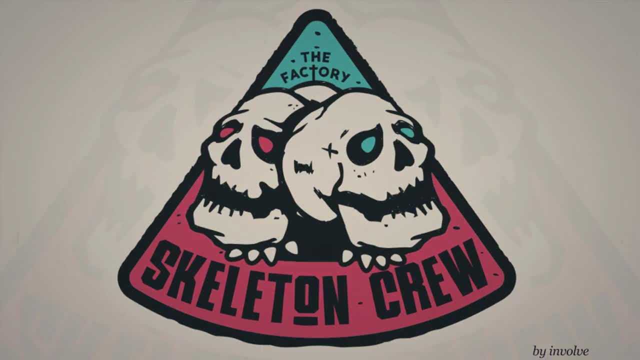 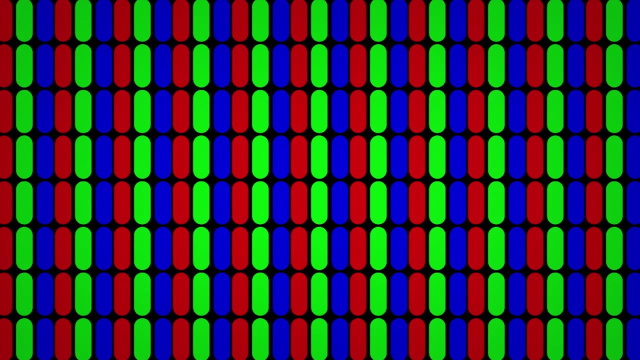 and computers. Today, RGB is the color mode to use if your design will be displayed on any kind of screen. If you take a very, very close look at your color screen, you can actually see the color split. That's because the light source within a device like a computer or a phone is part of the 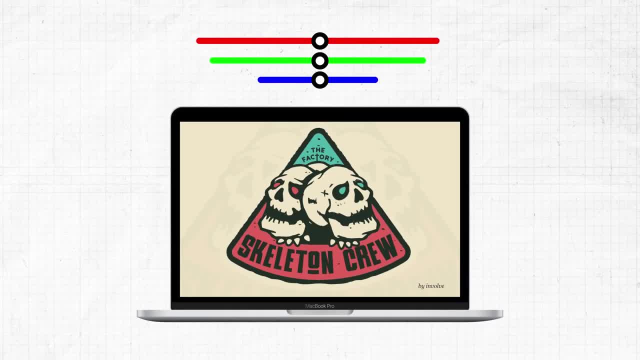 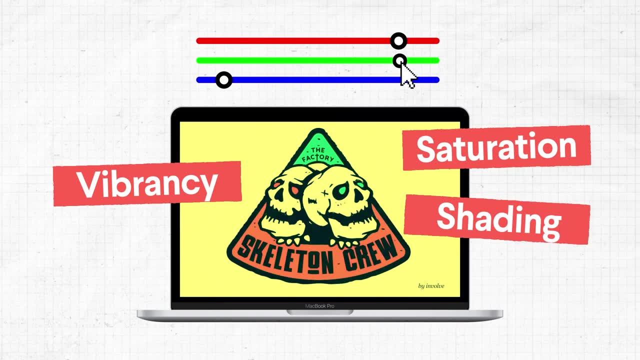 process that creates the color And it can change the intensity of each red, green and blue value. Designers can control things like saturation, vibrancy and shading by modifying any of these three source colors And, because it's done digitally, the designer can also. 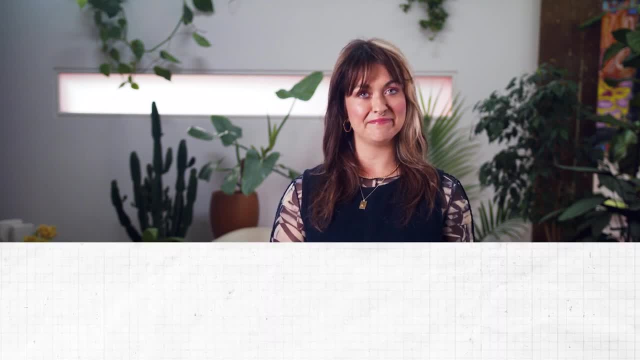 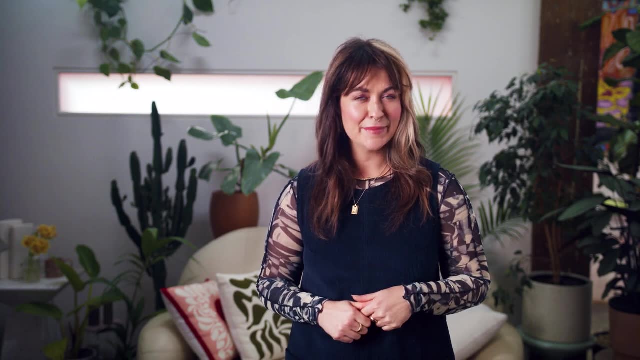 manipulate the light on the screen to create the color that they want. Now you know why it's important to use RGB in your design. It's because you can use it to create the color you want. Now you know what RGB is, but when do you use it? You'll need this color mode when your 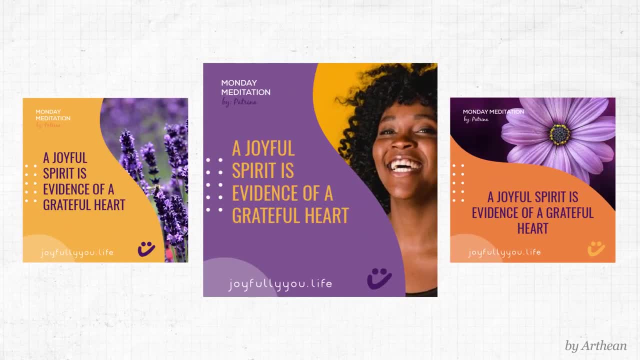 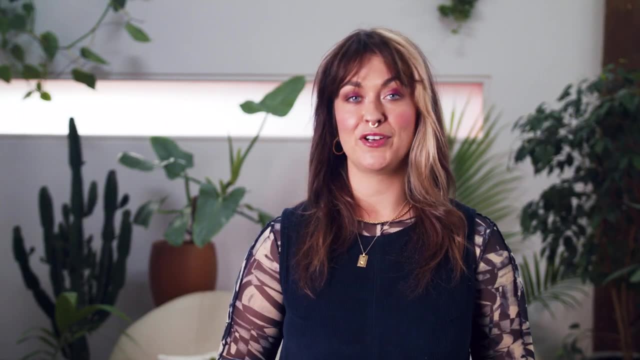 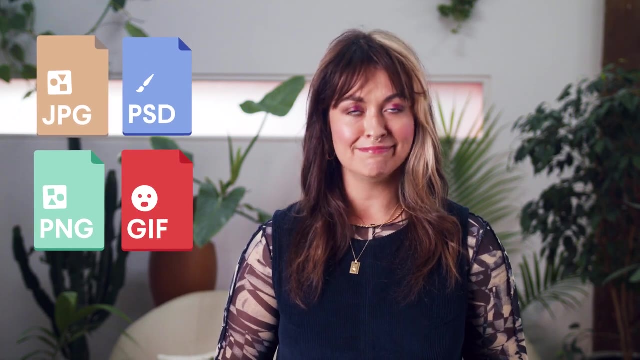 design project involves web and app design, social media posts, online branding and other visual content like this video you're watching. The best file formats for RGB are JPEG, Photoshop files, PNG or, everybody's absolute favorite, the GIF. What about CMYK? 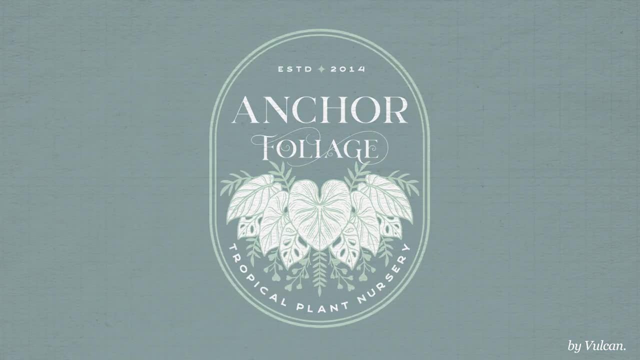 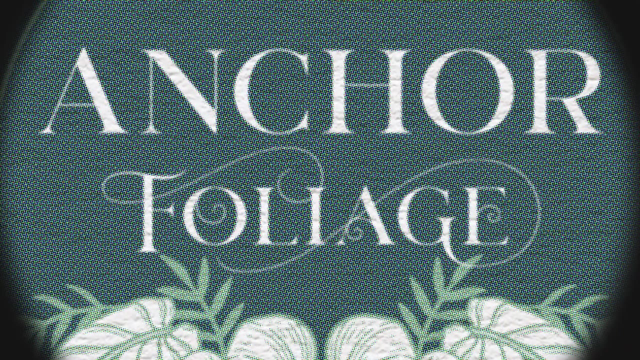 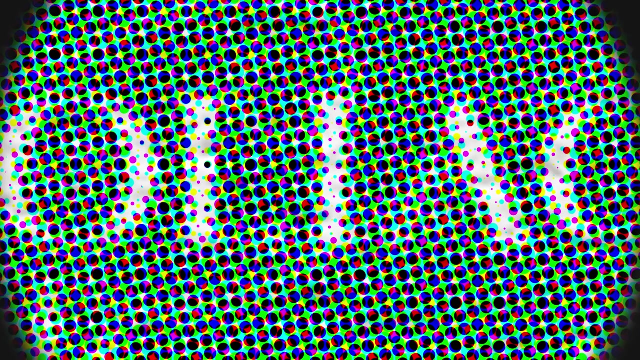 The acronym stands for the ink plates used in color printing, which are cyan, magenta, yellow and key. A CMYK printer layers tiny dots of these four colors in varying sizes to create an image. These dots are called halftones And if you take a magnifying glass, 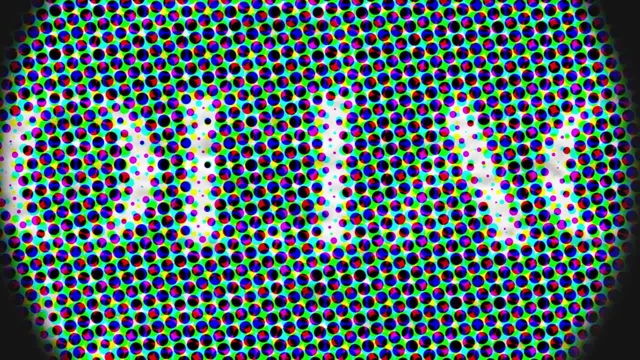 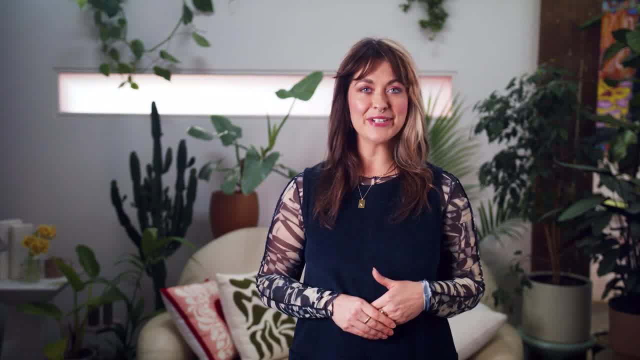 to a CMYK print, it would look like this: Fun fact: because CMYK requires the base paper to be white, CMYK printers don't actually print white. CMYK printers don't actually print white. CMYK printers don't actually print white. 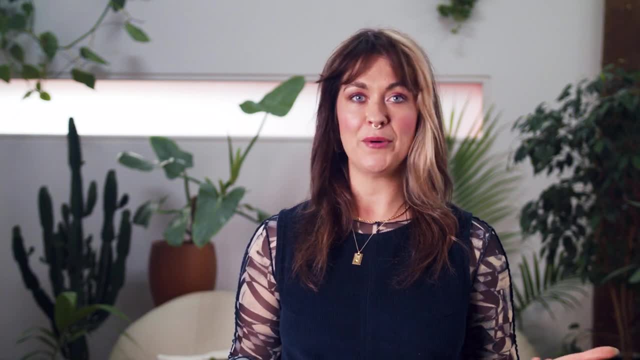 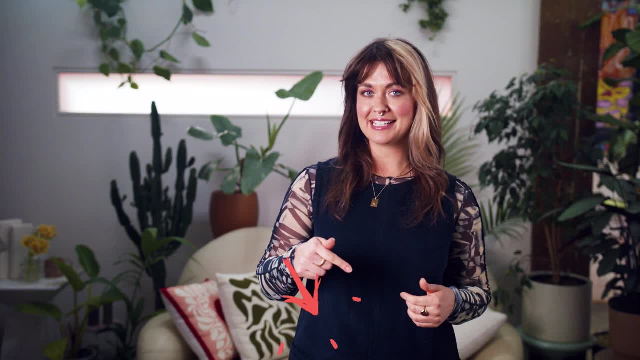 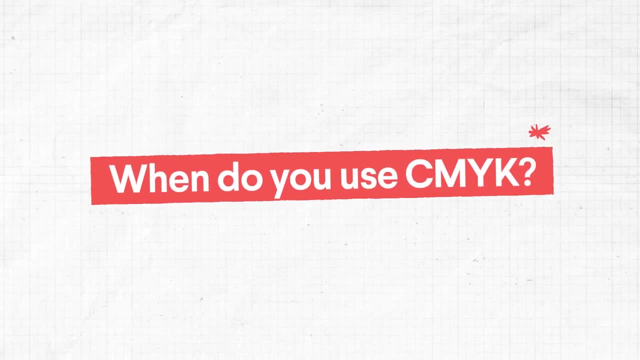 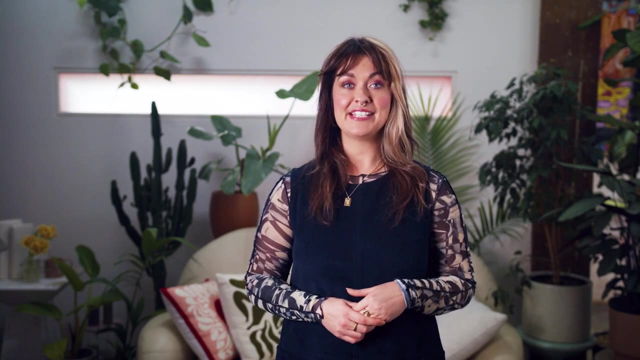 like how to change your color mode settings, click the link in the description box below. So when would you use CMYK instead of RGB? CMYK is for any design that'll be physically printed, ie not viewed on a screen.